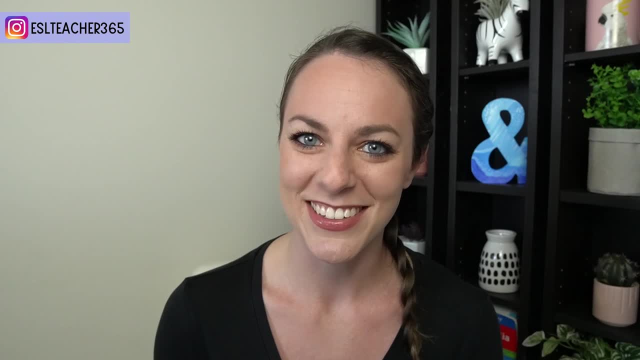 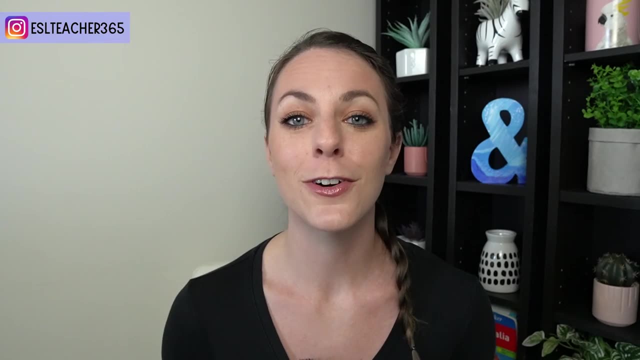 make sure to subscribe to my channel. All right, let's get back to the games. The second easy ESL game is Whisper Challenge. This game is perfect for all levels and is for reviewing vocabulary or working on vowel sounds. How to play the game is you're going to choose some vocabulary words? 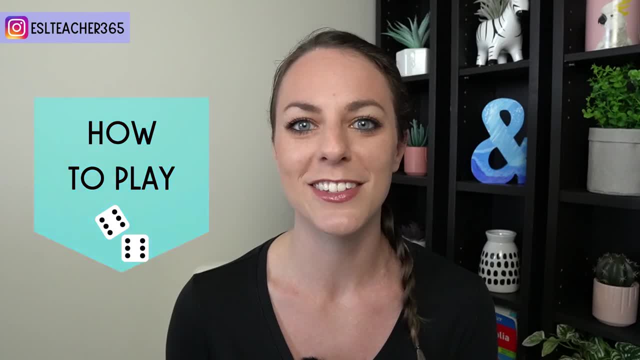 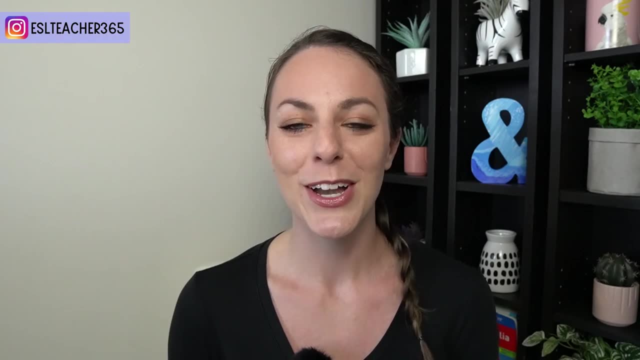 that you'd like your students to practice and write them on small pieces of paper. Then you're going to divide your class into two groups on opposite ends of the classroom. One group will be the whisperers and the other group will be the writers. So give each whisperer three different. 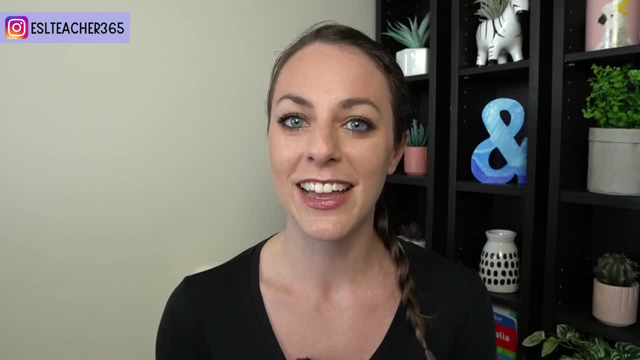 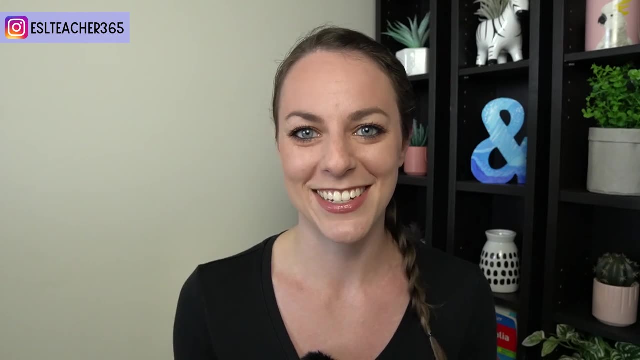 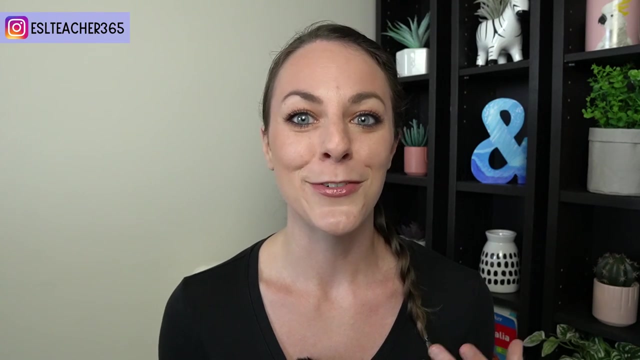 vocabulary cards and give each writer a piece of paper or a small whiteboard where they can write down the word that they think the whisperer is saying to them. So the whisperer isn't actually going to make any noise, they're just going to mouth the words. So, for example, 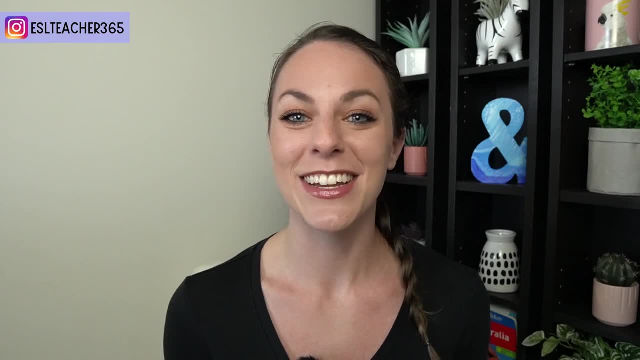 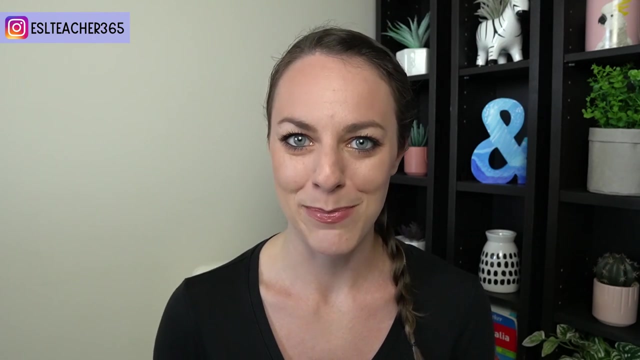 microphone, So they wouldn't make any sort of sound. they would just say to their partner and hopefully their partner understands and will then write out microphone or whatever they thought it was, onto their whiteboard or piece of paper. So some tips for this one, because we're not really used to. 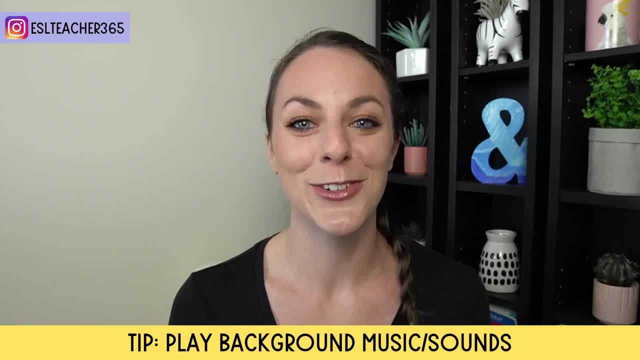 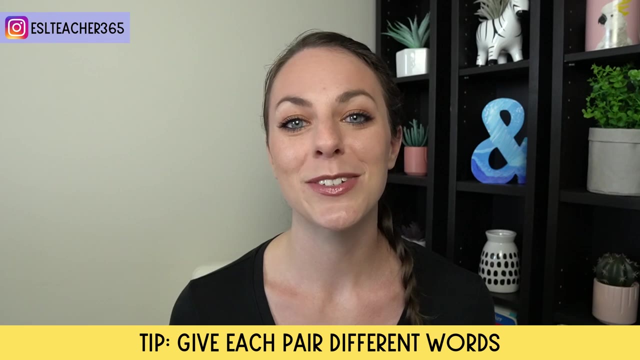 mouthing words. in our English class sometimes students do make a bit of noise, So I like to play random music or sounds kind of in the background to cover up any of these noises that can help their partner discover what word they're trying to say Additionally, you're going to want to make. 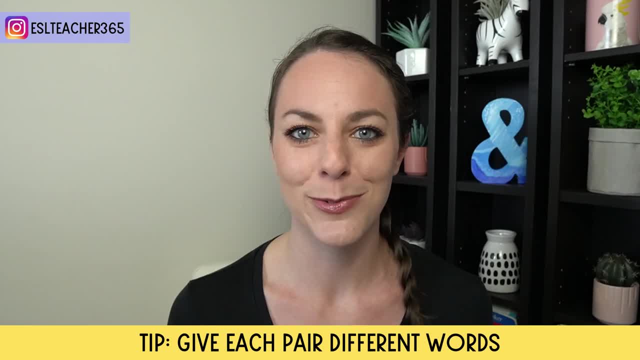 sure that any groups that are next to each other have completely different words, because otherwise they might be looking at someone else's words. So you're going to want to make sure that you're not looking at someone else and trying to. you know, use their the way they're saying it to help them. 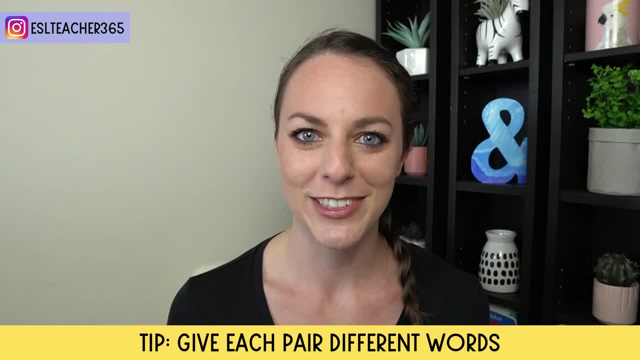 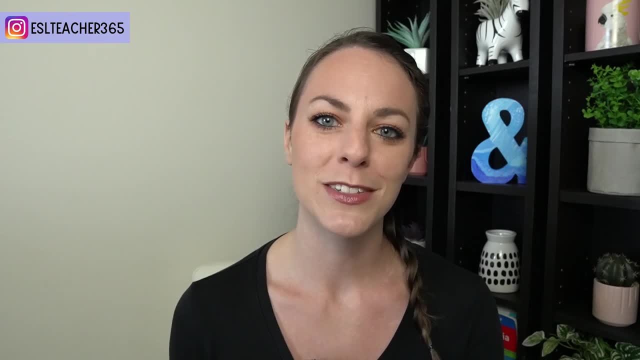 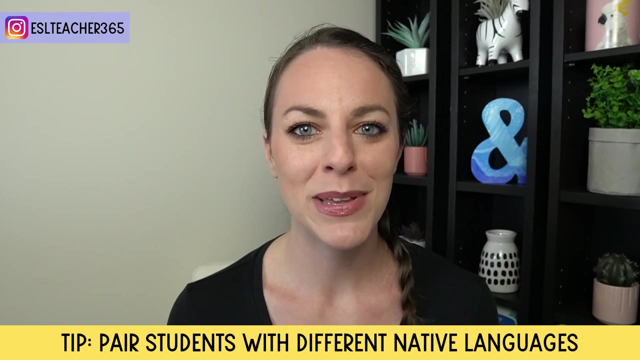 understand. So just make sure that all the groups have different words. You can switch after the whisperer has done three words and then the writer will become the whisperer, and vice versa. Another tip is, if you have a multilingual classroom, you're going to want to pair people. 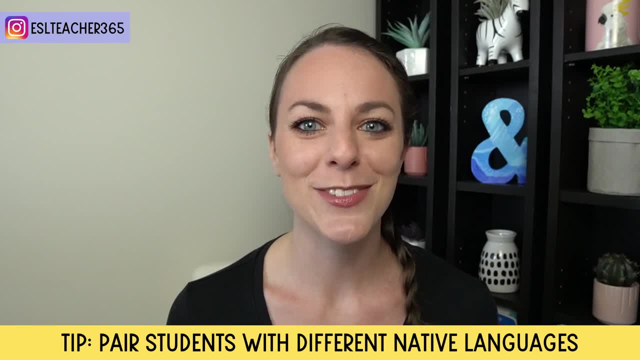 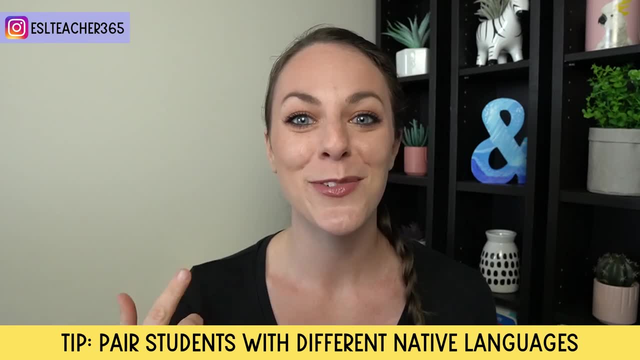 that have a different native language together. This makes it a lot harder. So, for example, a native French speaker with a native Japanese speaker, because of the way that they're going to form the words, because of their accent, it is going to be a bit more tricky than if you had two French speakers. 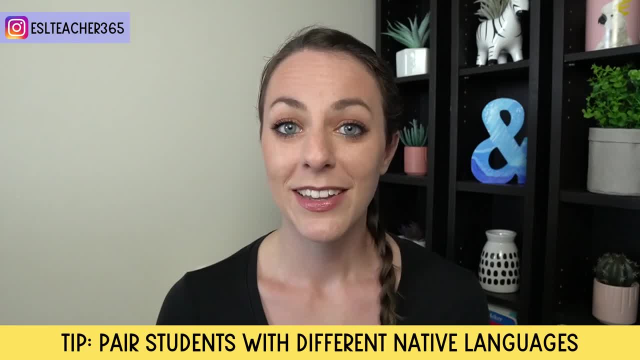 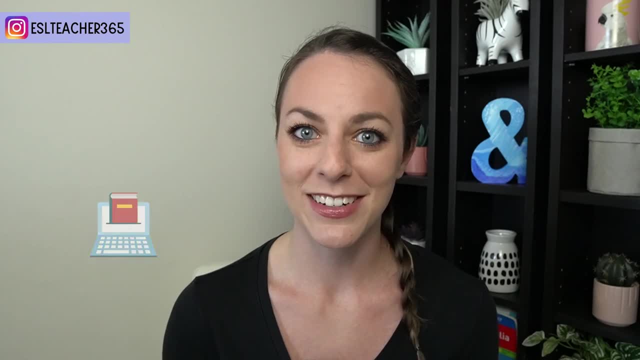 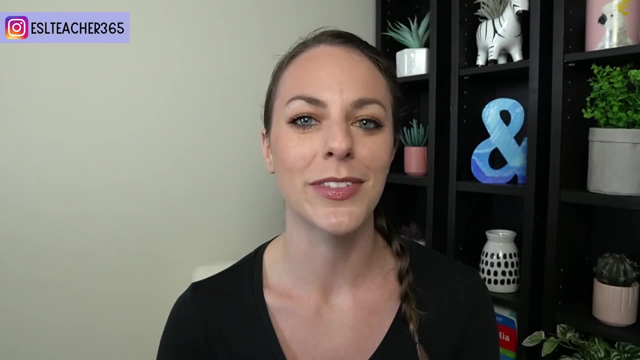 native French speakers trying to guess the words from each other. You can play this game online as well by spotlighting a student and sending them a word to say in the chat privately. Then they will say the word and the other students can either guess by writing down the word they. think it is, and then they can guess what the word is. If you have a multilingual classroom, you're going to want to try this out. Once you do check your notes and try guide yourself in either writing the words or by selecting the words in the optionses, If you have a multilingual classroom, 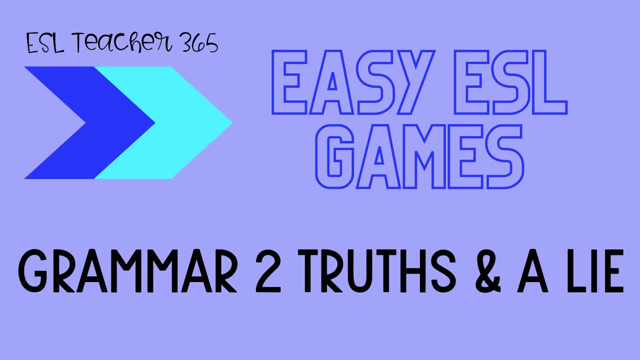 you're going to want to add a word or put the words in the search bar, But if you do, you can do that by typing your word and then in the fourth page you can add a word. The third easy ESL game is grammar: two truths and a lie. This is another ESL game that can. 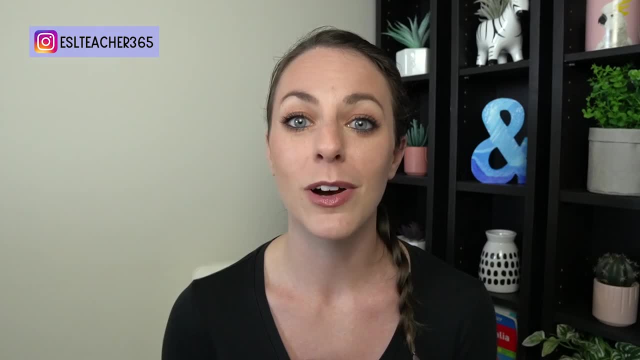 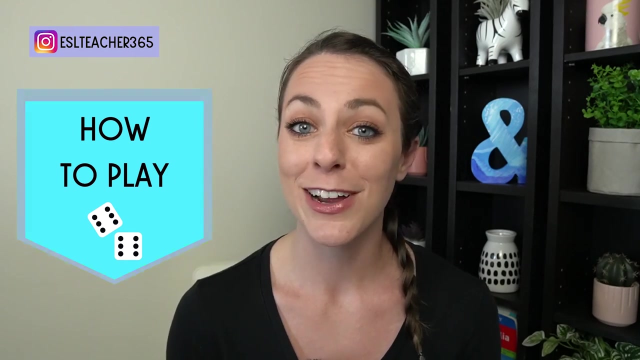 be used for all levels, depending on the grammar point that you want to practice or review. you can choose things like frequency used to present perfect conditionals and more How to play is. I like to model this activity for my students up on the board. First I write my name. 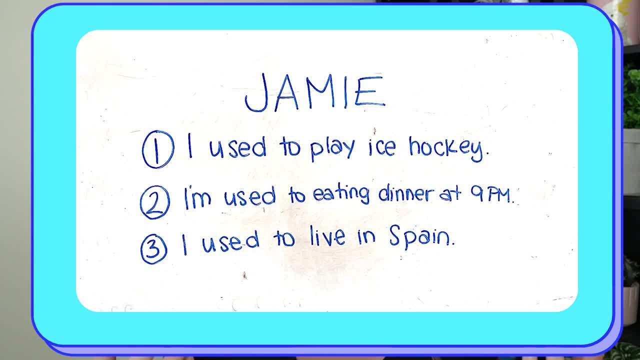 Jamie and I choose three sentences that are two truths and one lie, in any order and using the grammar point of my choice. In this case, I've used used to and be used to because I have students that confuse these two structures all the time. Then I'm going to have my students vote for which. 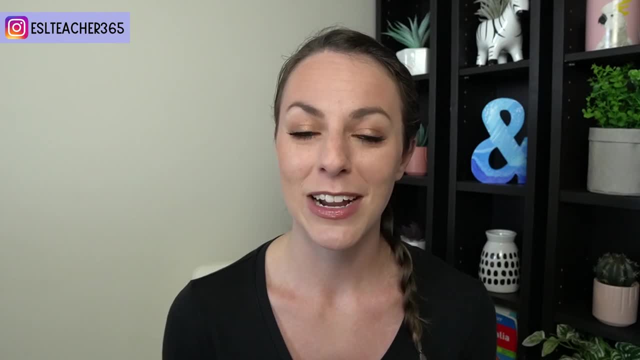 sentence they think is the lie. I will reveal if they were correct and allow them to ask me any additional questions. At this point I'll give each student a sticky note or they can use their notebook and ask them to do the same. Write their name at the top. write three sentences using the. 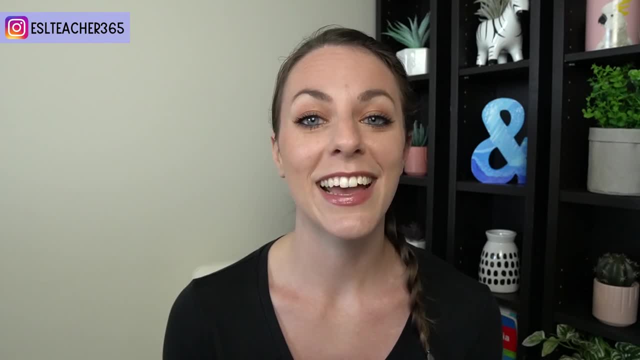 grammar point and choose one to be the lie and two truths. Of course it can be in any order, so your lie could be the first, second or third, but just remind them to make sure that it's only one lie or it gets very confusing. Then I'm going to have the students walk around and vote for. 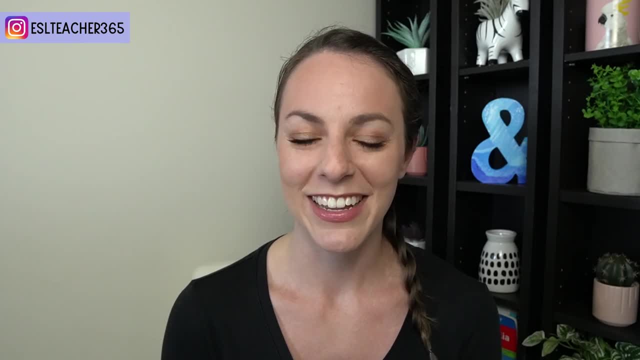 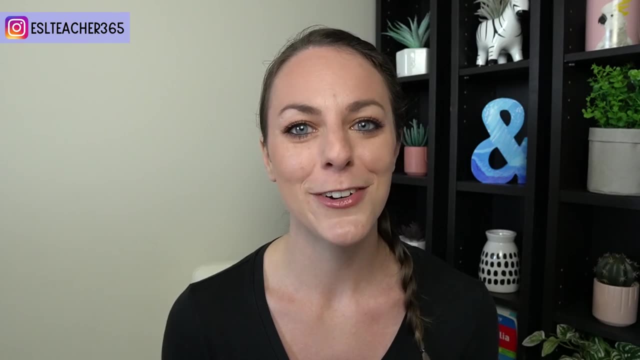 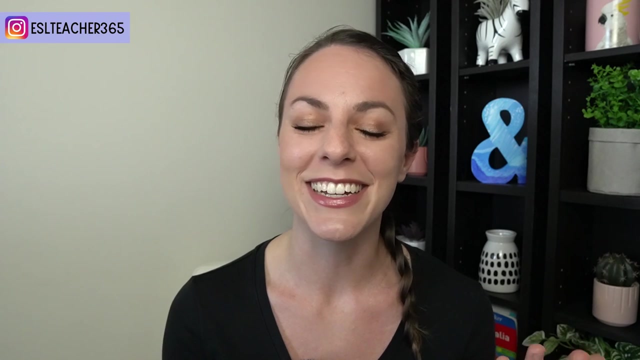 each person and see which one they think is the lie. You can also use this time to go around and check all of the grammar and make sure the grammar is good When everyone has voted. you're going to go, student by student, have them re-read their sentences to remind us of what we read and 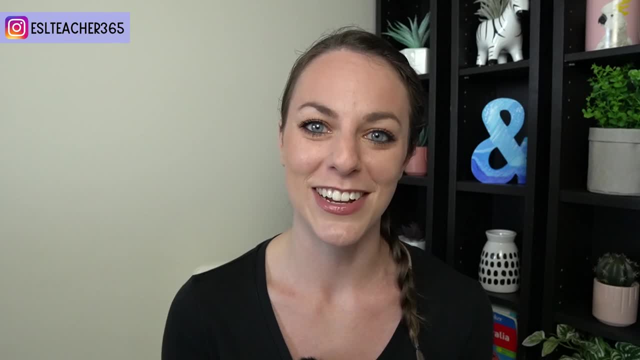 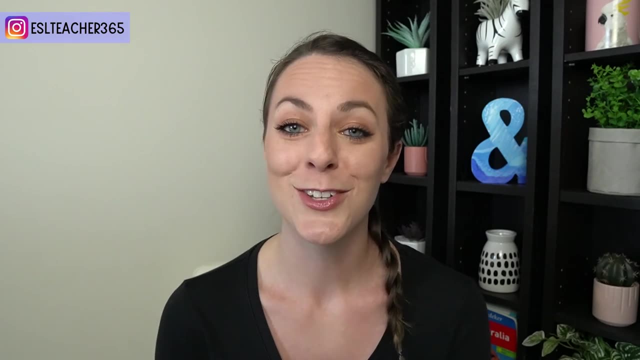 what they put down, and then we'll see if we guessed correctly or not. And if you have extra time, you can have your students ask any additional questions as well. You can also play this game in online classes by spotlighting one student, having them read their three sentences. 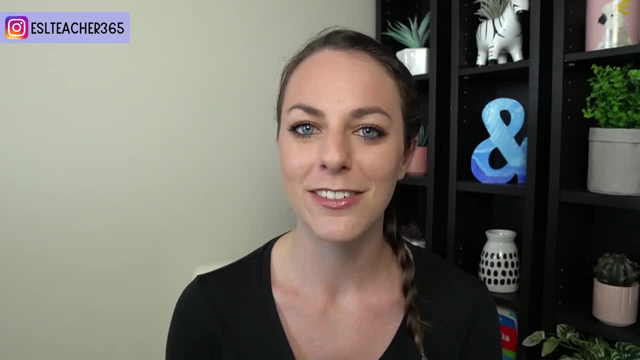 and then the other students can vote using the chat function, voting with a one, two or three, whichever sentence they believe was the lie. Then, once everyone has voted, the reader can reveal what the lie was and you can see if you guessed correctly or not. 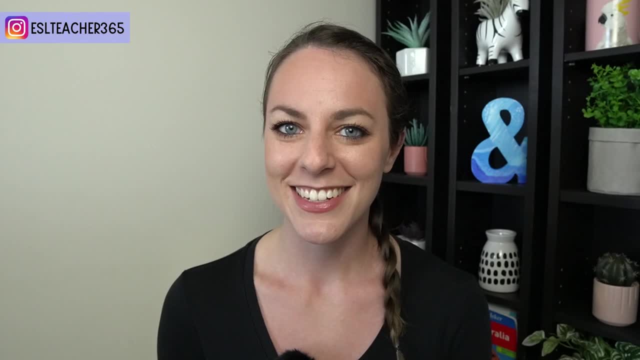 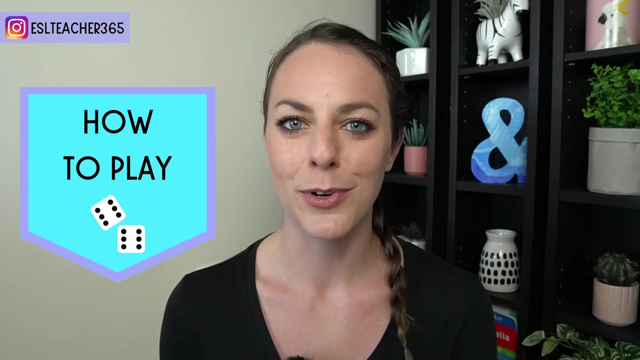 The fourth easy ESL game is Snowball. This ESL game is perfect for all levels and ages. Students will practice a specific grammar point, a verb, tense and asking and answering questions. To play the game, you're going to give each student a scrap of paper and write a question on the board. 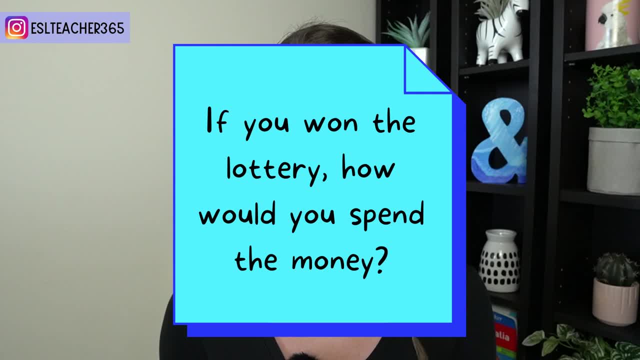 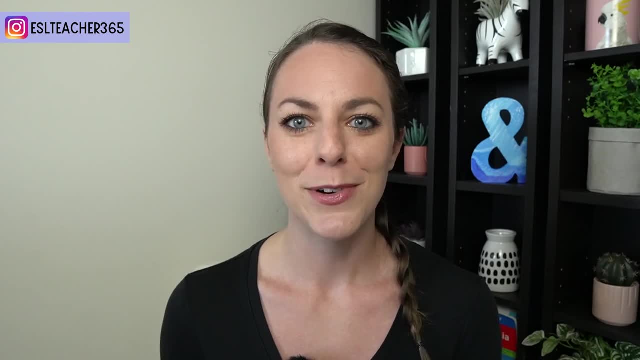 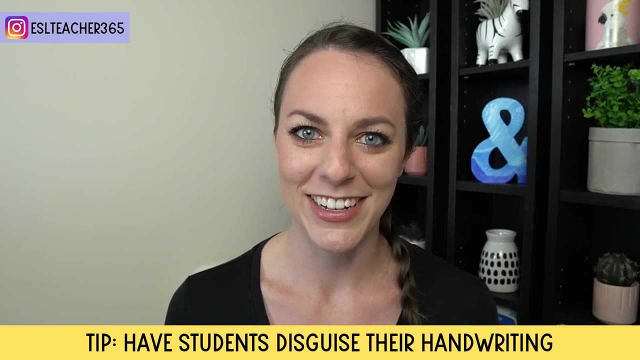 For example, if you won the lottery, how would you spend the money? Then ask your students to write just their answer on the piece of paper, so not their name. For example, they could write travel around the world, But if your students know each other well, have them disguise their handwriting. 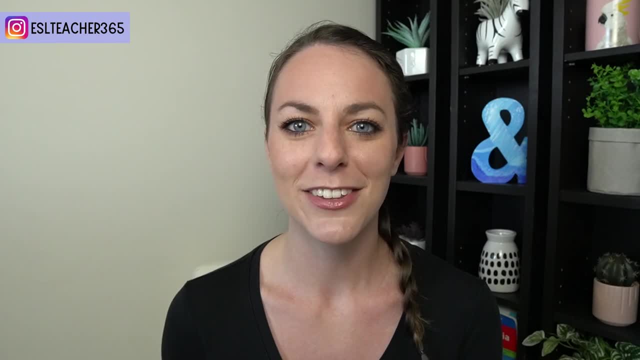 so it's not so easy To guess. then, when everyone has finished writing down their answers to the question, they're going to crumple up the papers into snowballs and, on the count of three, you can have them throw the snowballs at you, which can be fun, or you can put a target on the board and 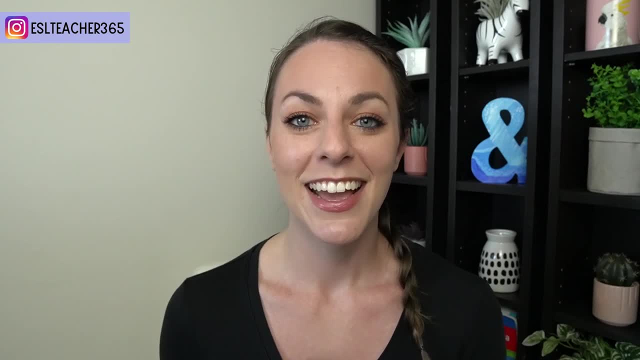 have them try and hit the bullseye. After they've done this, have all the students pick up one snowball each check to make sure that it's not their own, and then they're going to go around and ask the question to their classmates. So, for example, 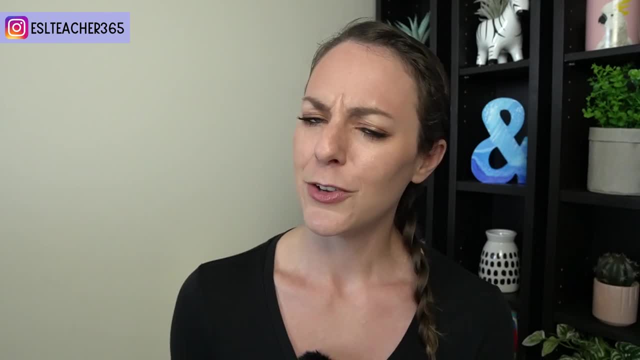 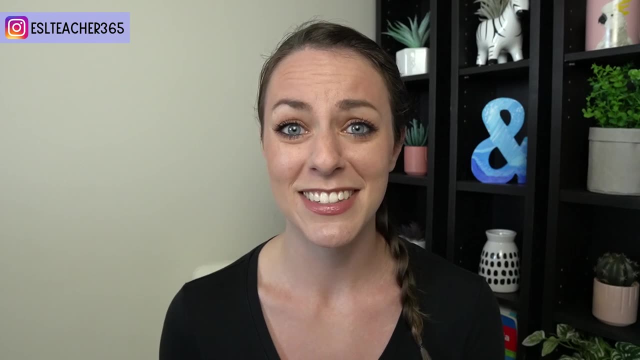 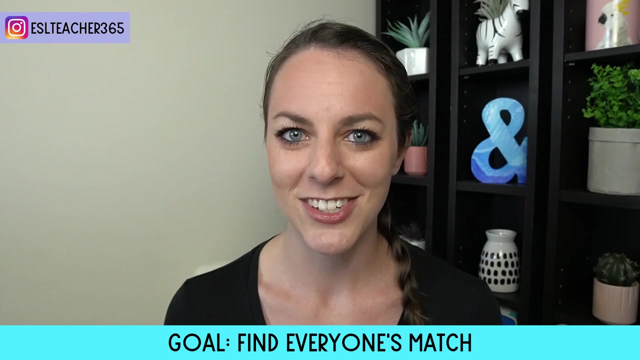 if the paper says buy a house, if you won the lottery, would you buy a house? If the person says yes, I would, then they've found their match. If they say no, I wouldn't, then you need to keep asking other students until you find your match. So the game ends when everyone has been matched up. 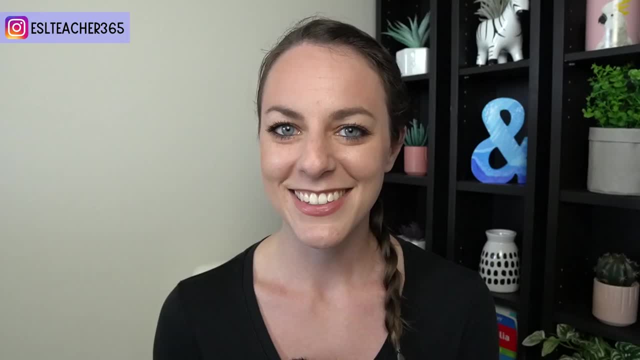 The fifth easy ESL game is Big Red Balloon. This ESL game is a mix of phonics and spelling practice and a bit of a riddling. This ESL game is a mix of phonics and spelling practice and a bit of a riddling. 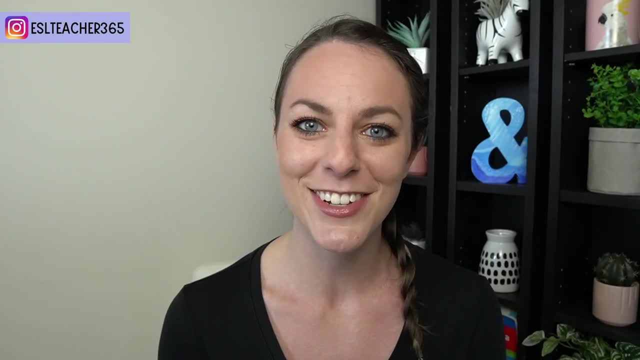 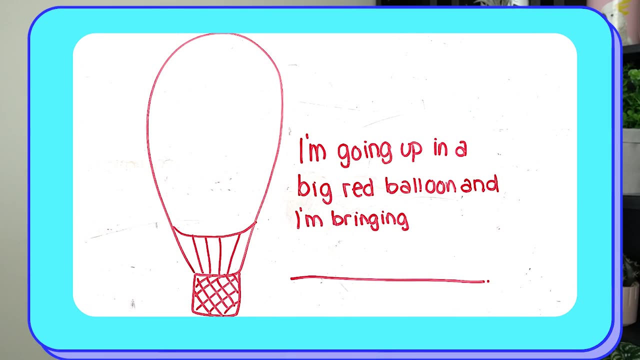 I first learned it at an English immersion summer camp in France called American Village. How to play the game is you're going to draw a red hot air balloon on the board and tell your students I'm going up in a big red balloon and I'm bringing a, and then say an item. 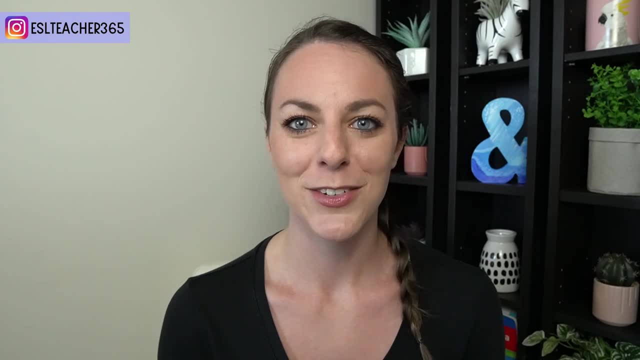 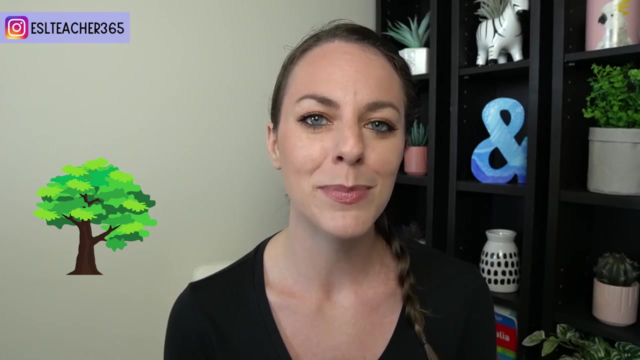 based on whatever spelling or sound pattern you have picked out. So for this example, we're going to use double letters. So I might say I'm bringing a tree. Then you're going to ask a student, hmm, what are you bringing? and have them repeat the whole thing. So I'm going up in a 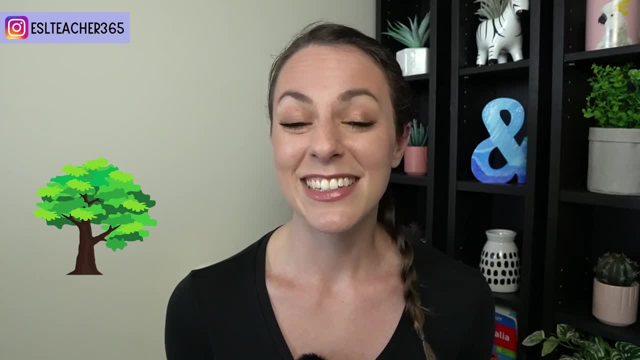 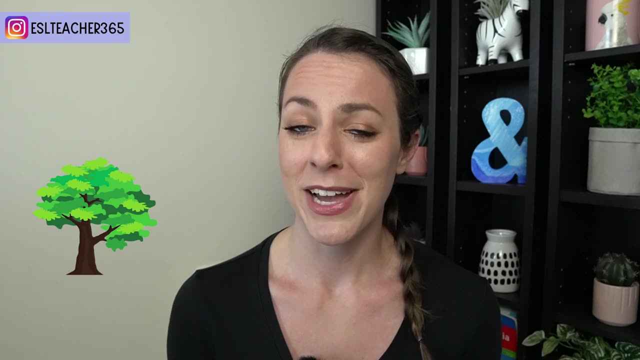 big red balloon and I'm bringing a. At this point they're not really going to know what's going on, so they could say anything. So I'm bringing a suitcase, But you know the pattern. so you're going to say no, you're not, you're not bringing a suitcase, I'm bringing a tree, but you're not. 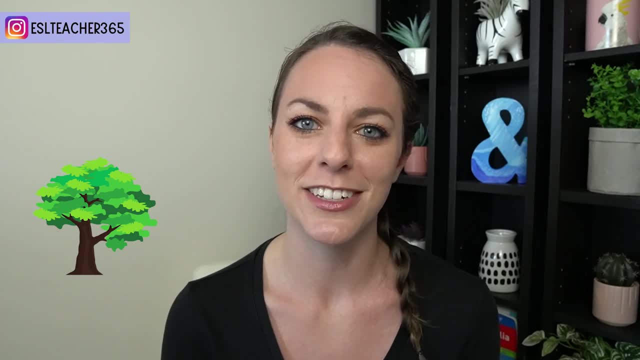 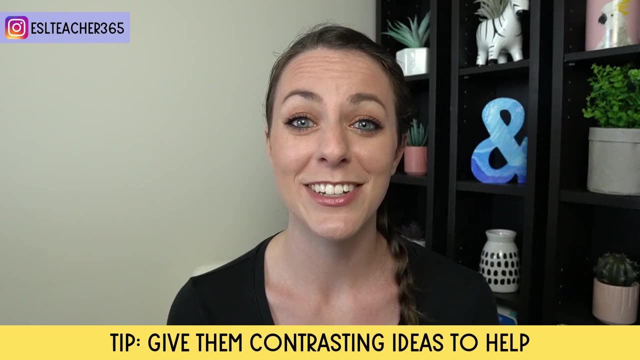 bringing a suitcase. Then go through your other students and see if they can guess. At this point you're just guessing random things. If your students are completely frustrated, you can give them some help. So, for example, I'm bringing a spoon but I'm not bringing a fork, So they can. 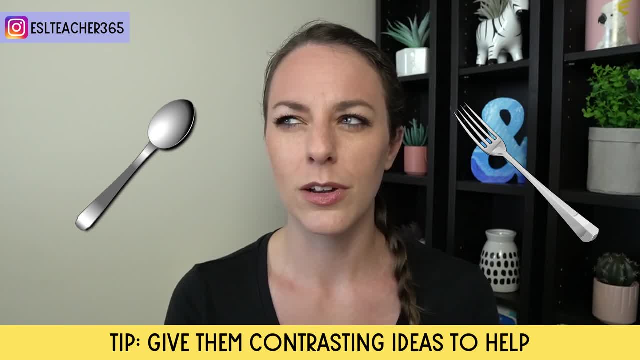 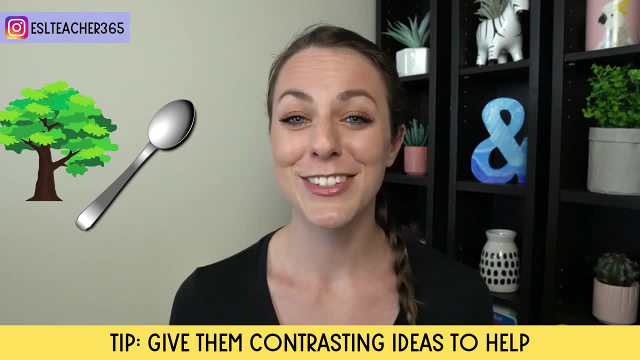 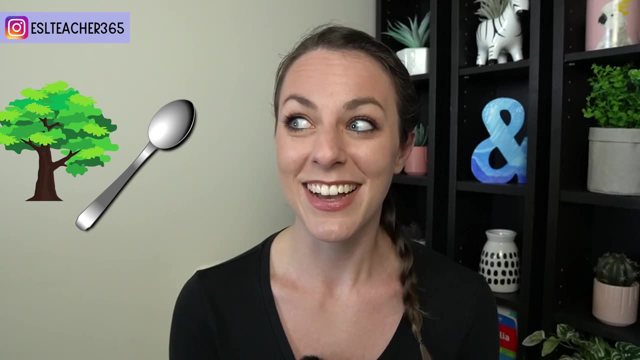 start to think: hmm, why is she bringing a spoon but not a fork Spoon tree? maybe it will start to click with one or two students. If one or two students start to kind of figure it out, you can have them give some examples of things that they're going to bring and you'll start to say: yes, 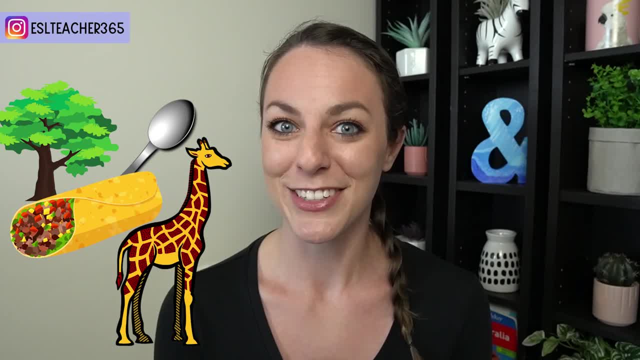 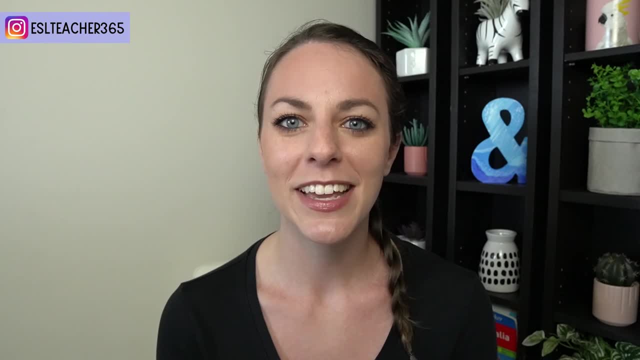 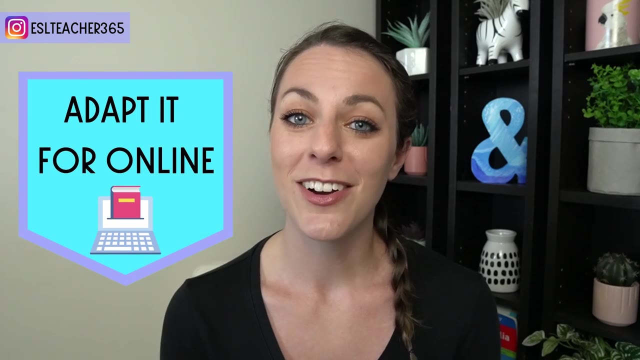 you are bringing a giraffe, You're bringing a burrito, that's right. It'll probably drive the other kids crazy, but eventually you can explain what the pattern was and continue the game with a new vowel, sound or pattern of your choice. Because this game is mostly oral, you can also play this online. 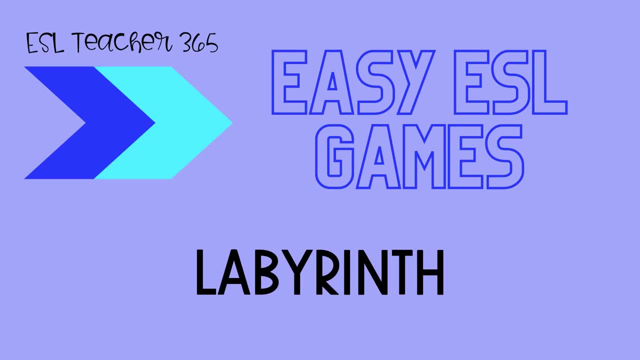 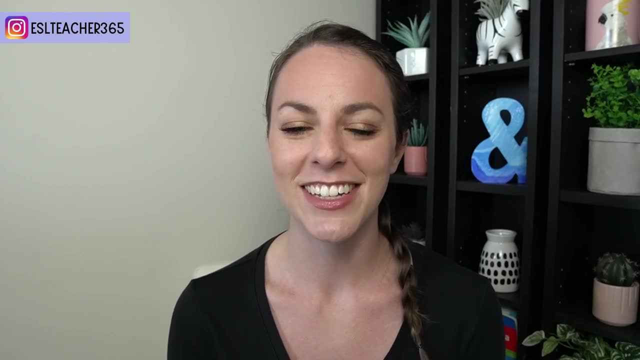 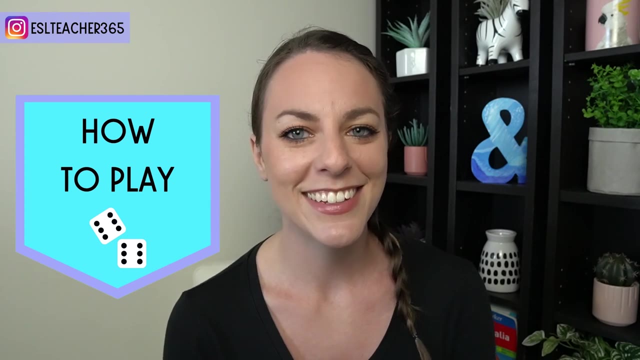 and it's a really fun, quick icebreaker or warmer. The sixth easy ESL game is Labyrinth. If you're looking for a review game that also practices pronunciation, then Labyrinth is a great choice. How to play the game is you're going to choose 24 vocabulary words? In this example, I'm 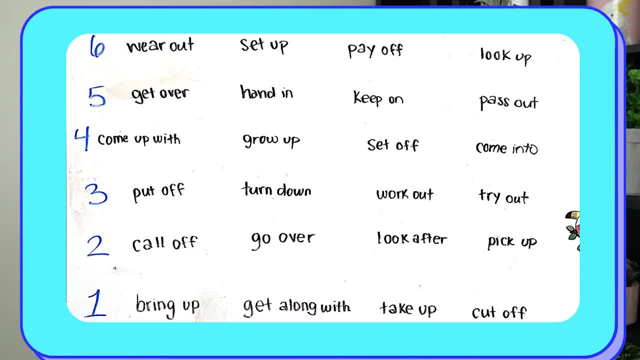 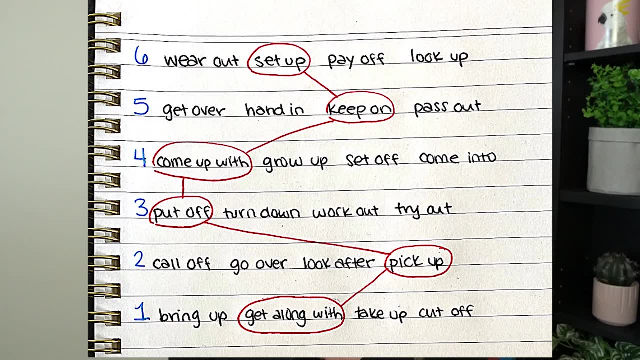 using phrasal verbs. So you're going to put them in rows with four words per row for six rows. You're going to write this up on the board and you're also going to make a copy for yourself on a piece of paper. Then you're going to select on your paper one word from each row, going from the bottom. 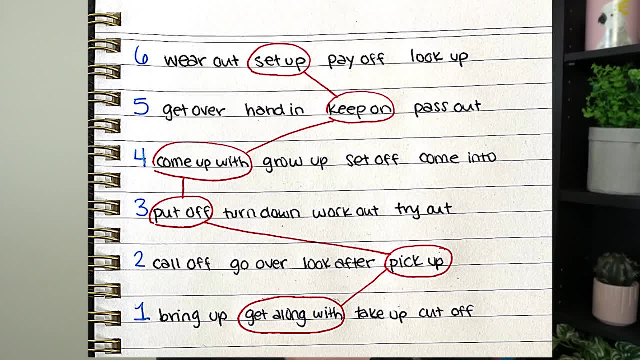 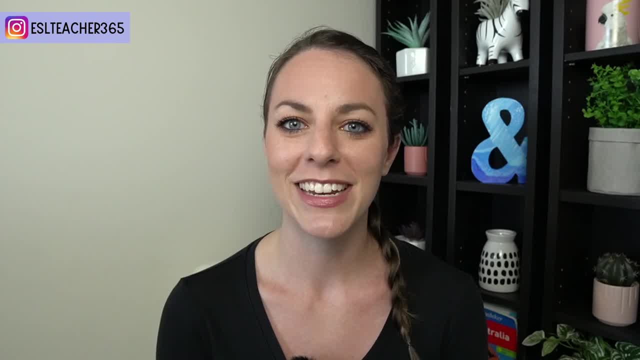 to the top to create a bit of a maze or labyrinth. Next, you're going to divide your students into groups of two or small groups and let them know that they need to guess the correct word in each of the six rows, from the bottom to the top, and 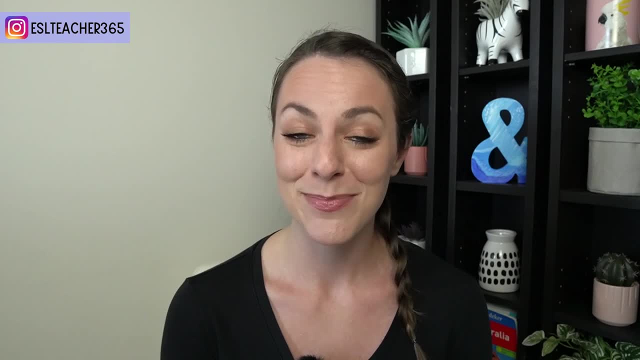 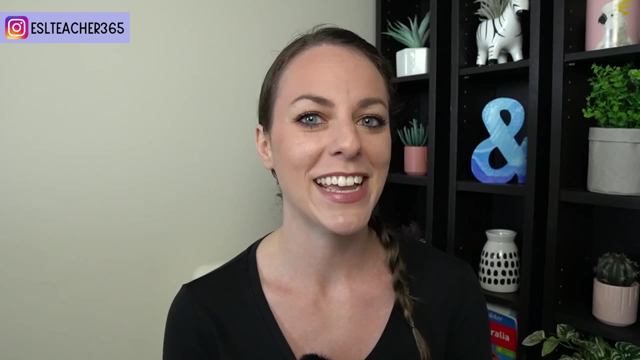 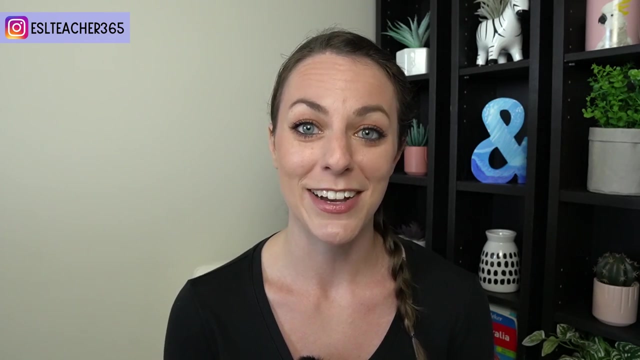 when they do this, they are the winners. But because we're reviewing and practicing pronunciation, they need to pronounce all of the words correctly and they need to give you a definition. The first group is going to choose whichever word they think is the correct one that you have chosen. 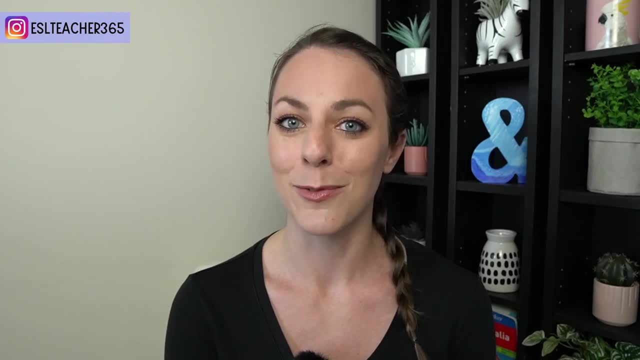 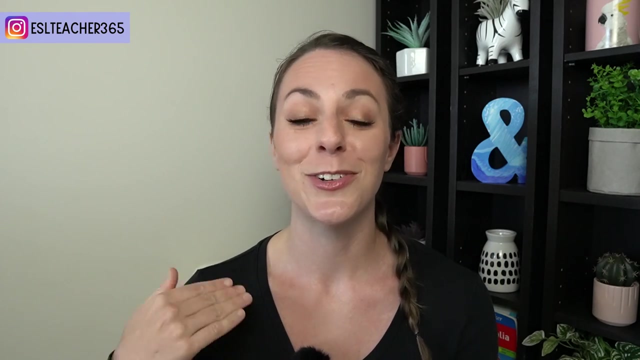 If they are correct, then they need to pronounce it properly once again and give you a definition, and they'll keep moving up until they make a mistake. If it wasn't the word, their turn is over and the next group has to start from zero. This is a great way to practice repetition. 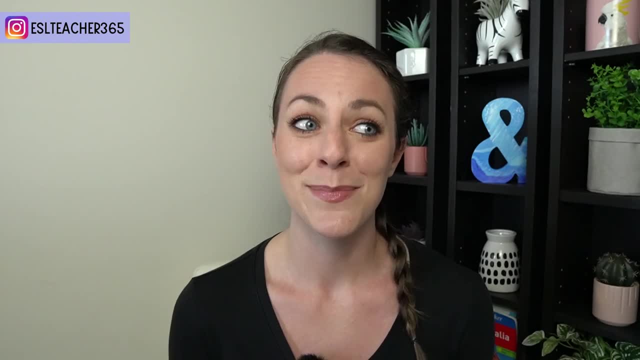 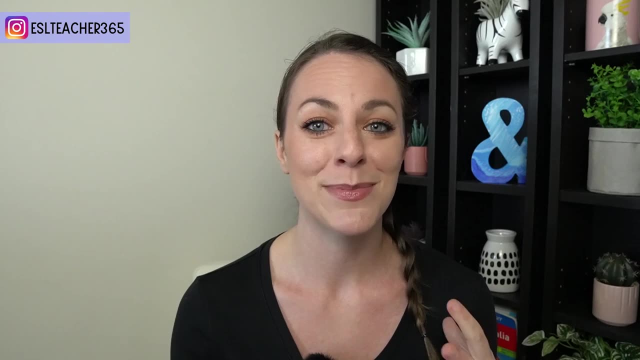 They have to listen to the other groups and pay attention. They might want to copy some of the definitions they're hearing from the other groups as well, as well as the pronunciation. So the first group is going to choose which word they think is the correct word. So this just keeps. 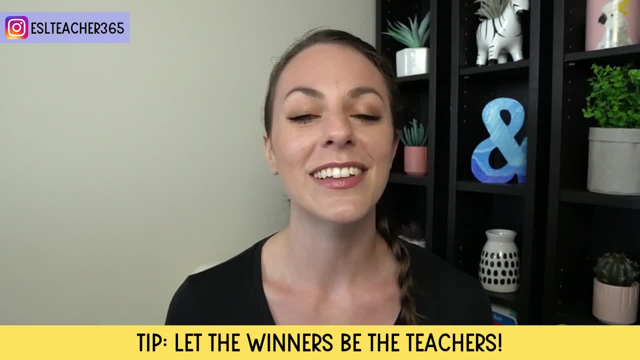 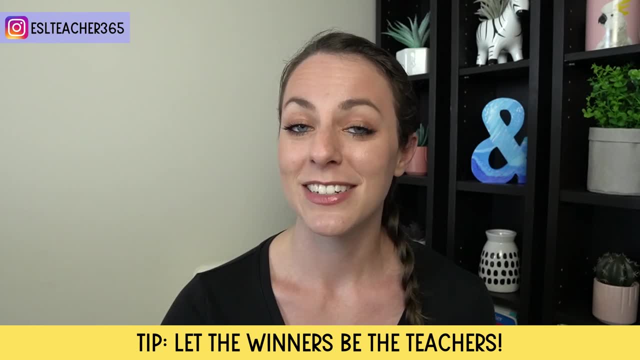 everyone really interested. Finally, when you have a group that has guessed all of the words in your labyrinth, I like to allow them to become the teachers So they can come to my piece of paper, use a different color, choose a different path through the labyrinth, and now they are in charge. 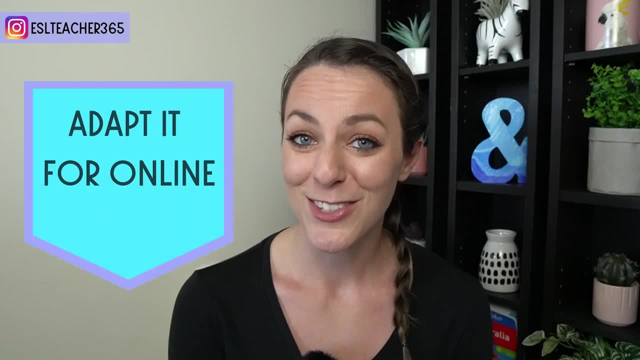 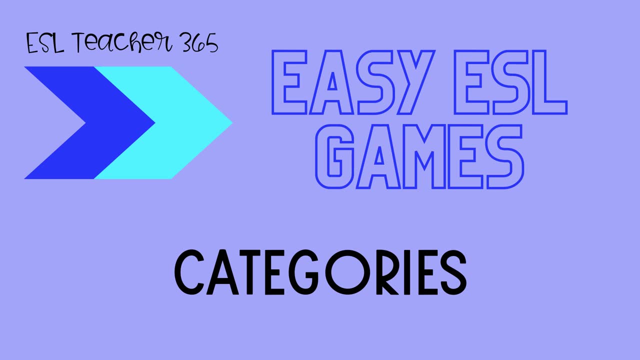 of the game and I'm just there to make sure that the definitions and pronunciation are correct. You can also play this game online by using the whiteboard function. Another easy ESL game is categories. This is a fast-paced vocabulary game that's great for all. 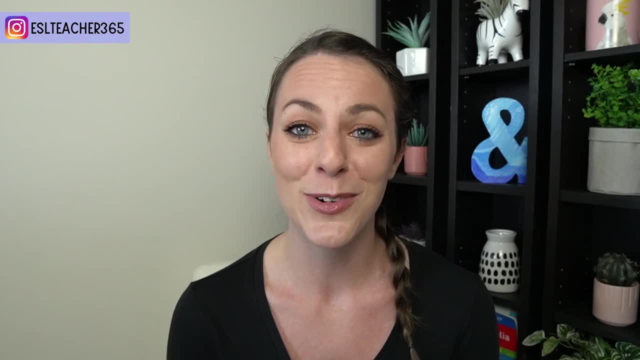 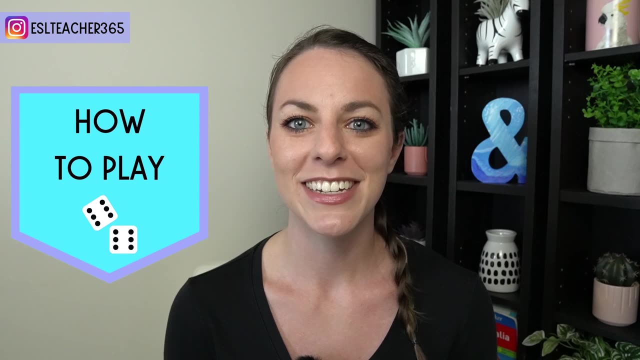 levels and can be used in person or online because it doesn't require any materials. How to play? is you're going to choose a category to start with, For example, colors? Each student needs to say one color and they cannot repeat any of the colors that have been said by the other.